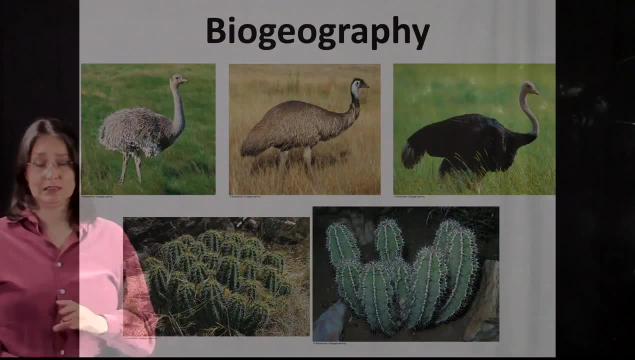 and Australia, together with also India and even Antarctica, were part of a much larger southern continent called Gondwana or Gondwana land. We'll go to a map of that in a moment. So now we know that these birds are actually related to each other. 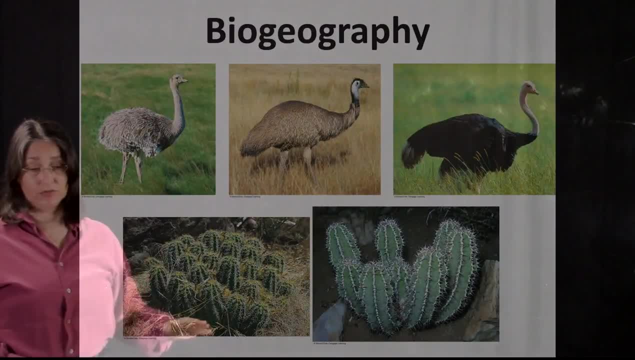 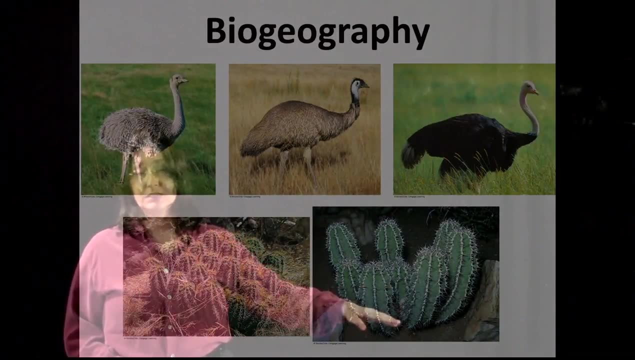 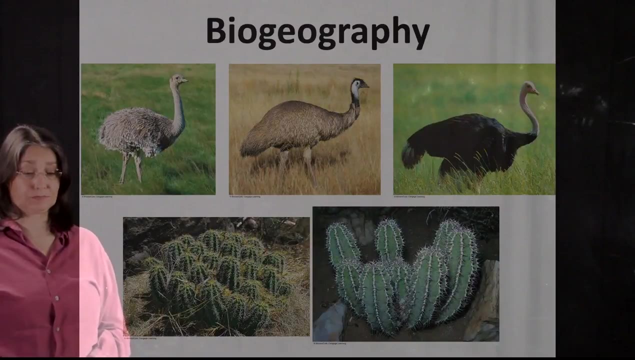 But if we look at these two plants at the bottom, so a cactus here on the left and a euphorbia. So even though this plant from southern Africa is called milkweed barrel cactus, it's not a cactus, And now we know that. all the cacti. 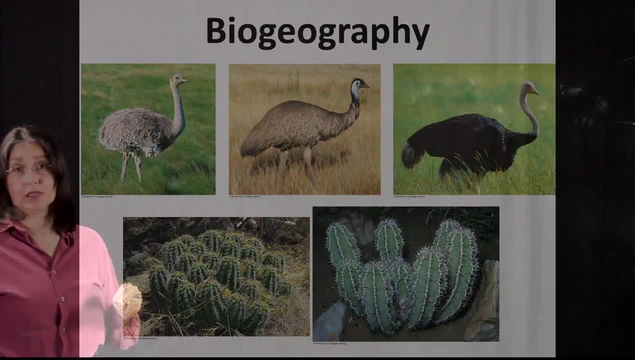 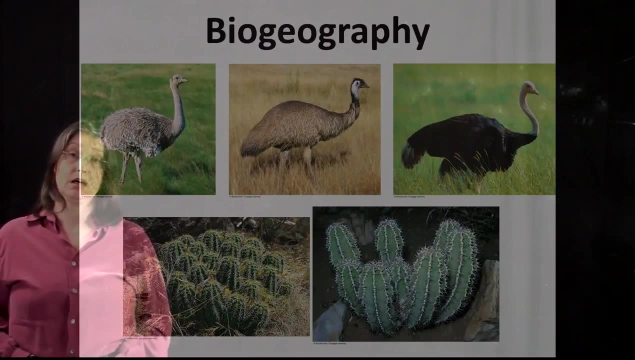 inhabit only the Americas, North America and South America. So cacti, the family of cactaceae, has evolved probably only after the inception of the Atlantic that separated Africa from South America. So they are not related, Even though they are both flowering plants, so they have that. 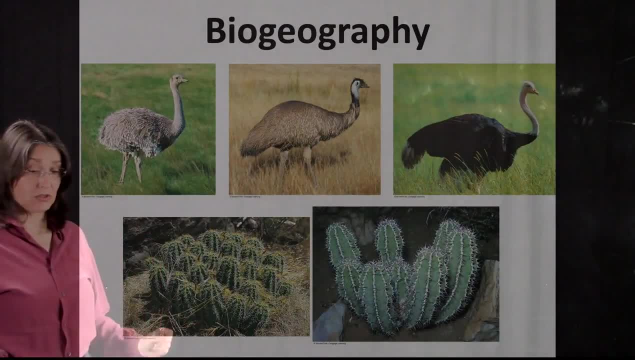 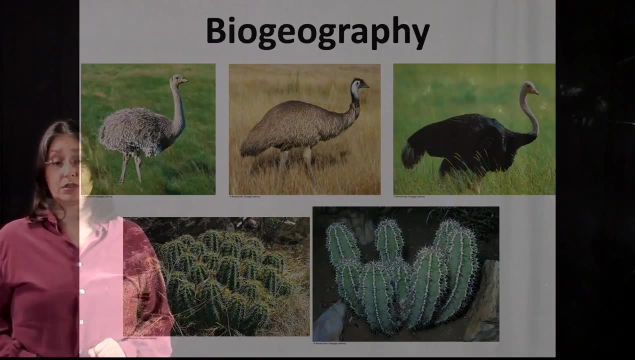 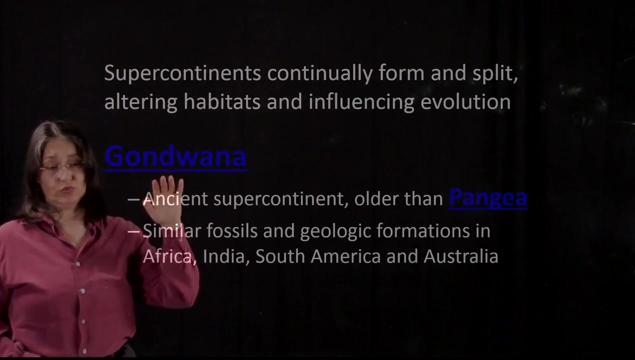 common descent or common ancestors. excuse me, they're actually from two different families and their adaptations are different. So this is an example of convergence to adaptation to the same dry habitat. So speak about super continents such as Gondwana, or Gondwana land, and Pangea. 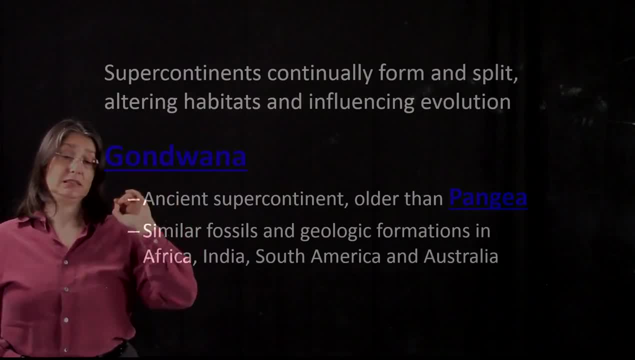 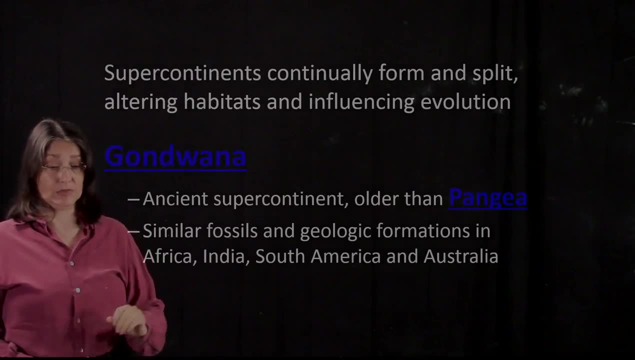 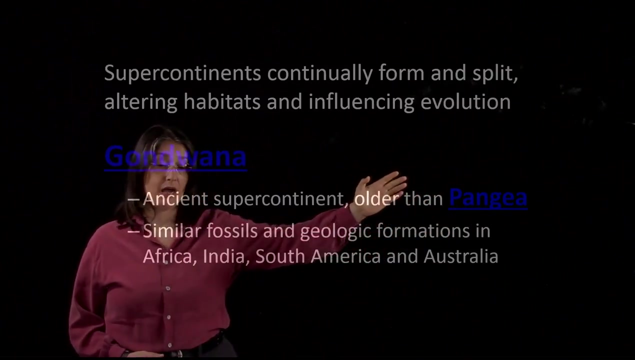 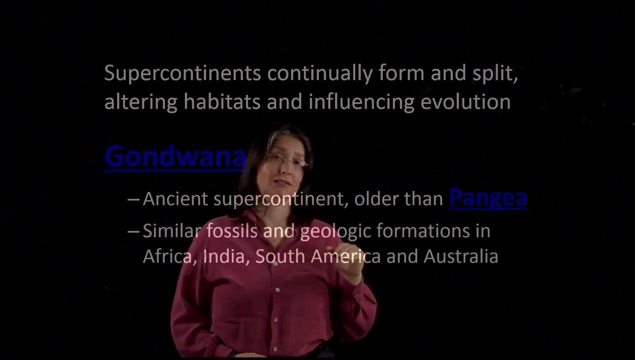 Now we know that about 500 million years ago the southern landmass formed Gondwana And then, sometime later, Pangea was formed. That literally means all earths. Gea or Gaia was the mother earth in Greek, and pan means all, So Pangea is only about 270,. 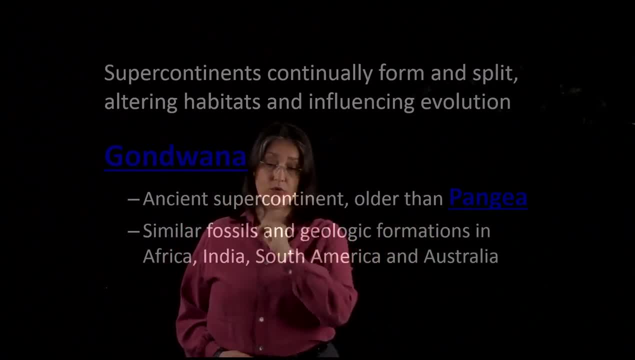 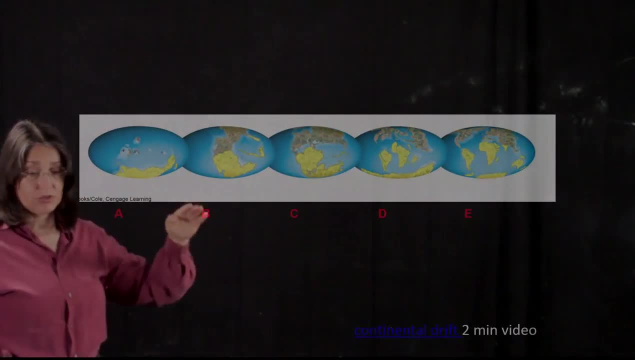 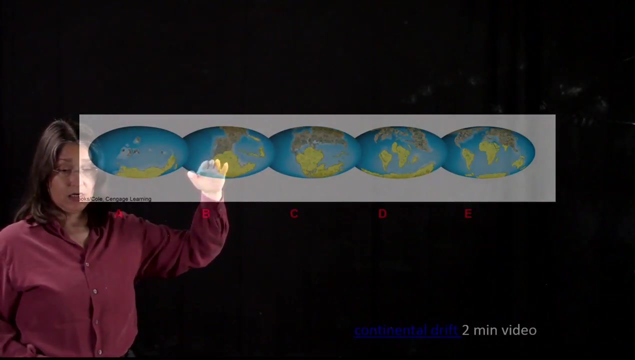 so less than 300 million years old, when Gondwana land it's 500 million years old. So let's take a look at this map just from your textbook. So here in yellow you can see the Gondwana land about 500 million years ago, And then you can see Pangea. 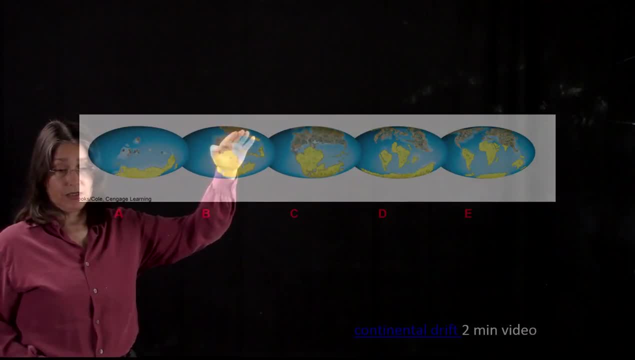 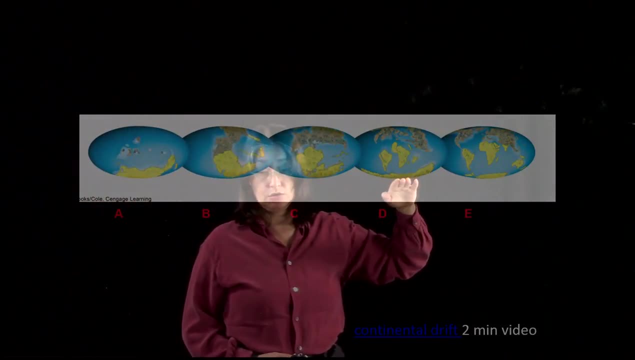 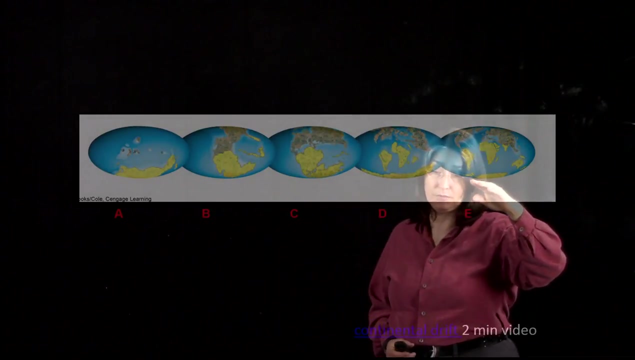 that includes North America and Eurasia, right here And then. now we can see how they differentiated today. So this is before 180 million years ago, when the Atlantic divided South America from Africa, And they keep on moving away from each other at a rate about two centimeters plus a year. 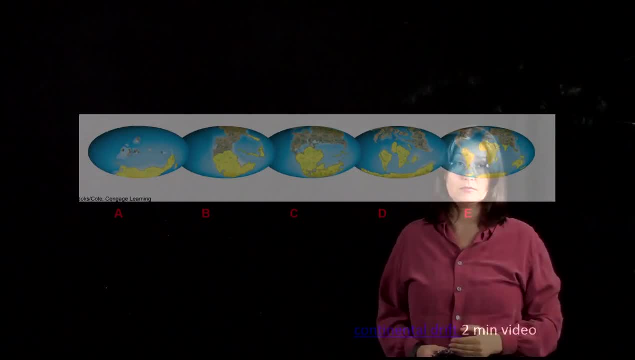 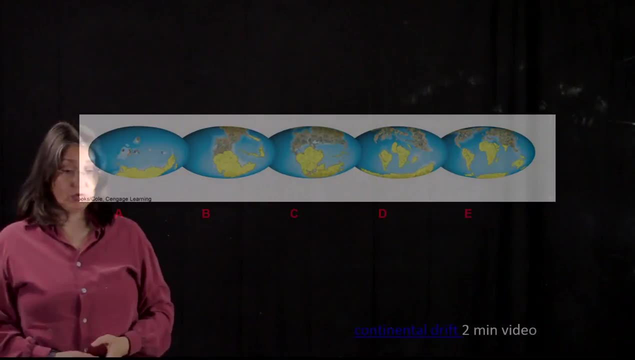 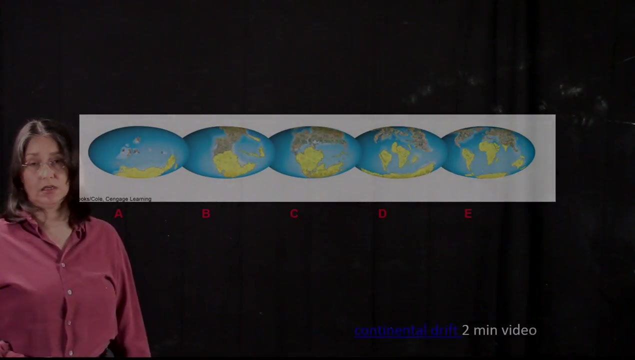 So the Atlantic keeps on expanding while probably the Pacific keeps on getting smaller, So landmasses themselves were not static, so they moved around. And please click on this link. There are several other links and your textbook has different ways of thinking about this continental mass drift and shifts and bumping to each other. 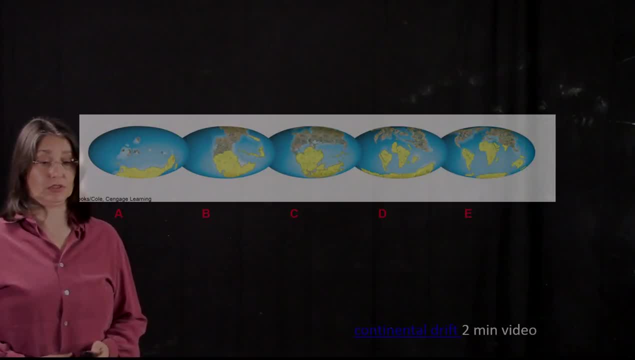 And separating from each other, which led to species evolution adapting, either coming from a common descent from Gondwana land, like those three large walking, flightless birds, versus the two plants that I showed you, one from the Americas and the other one from Africa. 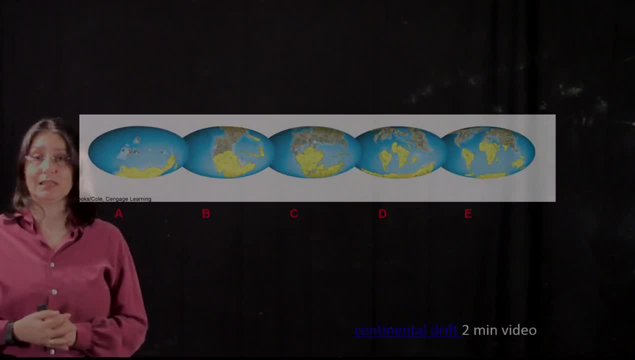 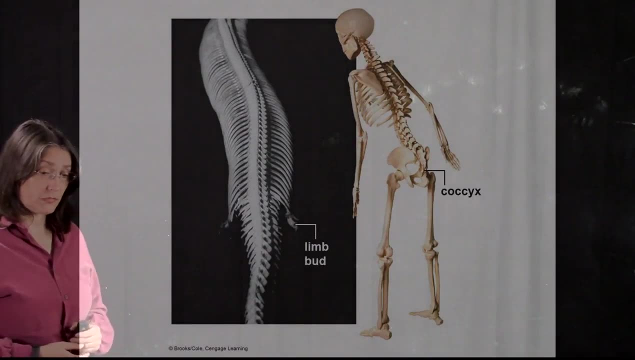 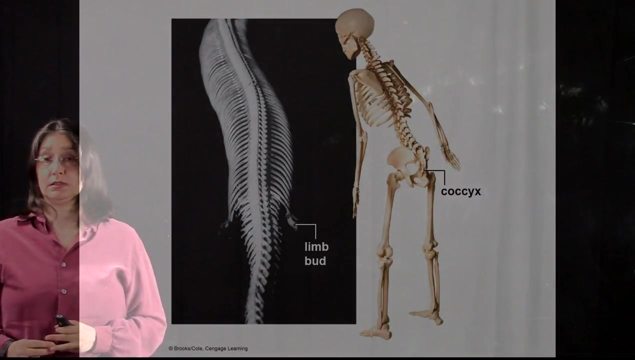 that look alike. but they only look alike because they responded to the same environmental pressures, not because they are from the same group. So, moving on to the next area of naturalist explorations that led us to our thoughts of evolution, The next one to consider is comparative. 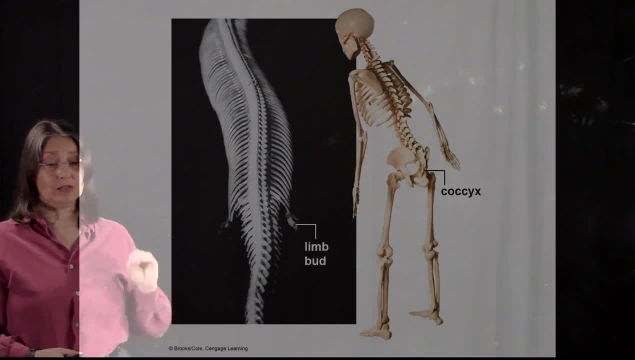 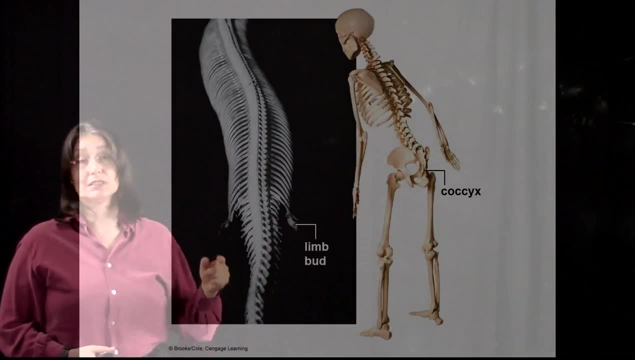 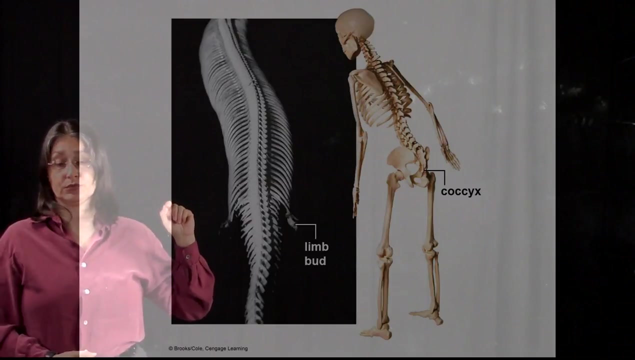 morphology, And in this case we can even look to comparative anatomy. So what you see here again straight from your textbook, you can see a human skeleton versus a snake skeleton. So right away you can see that we have way less, way fewer vertebrae and way fewer ribs. 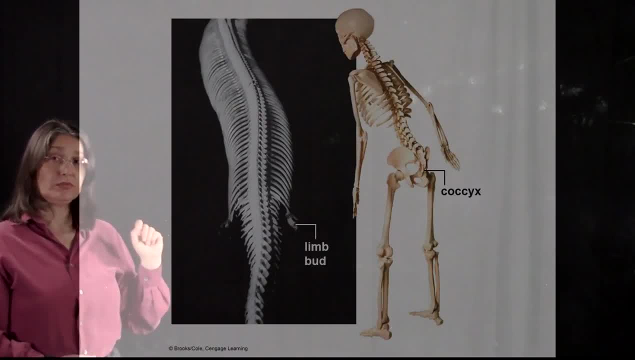 But we still have a tailbone. So even though most humans are not born with a tail- and when they are it's removed really early on- we do have this vestige. So the example here refers to vestigial and the same here is for ancient structures that are no use anymore. So Lamarck was right in this. 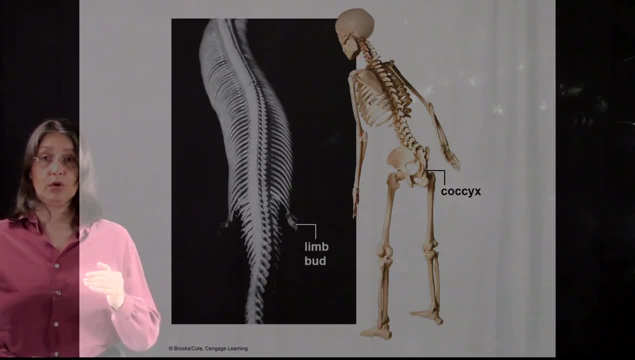 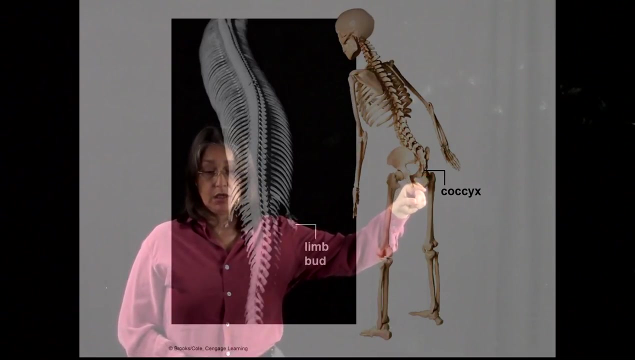 perspective: what you don't use, you lose. So, comparative to a more primitive, so earlier species, such as monkeys, that could use a tail for balance, we don't need it. So we do have a coccyx, which literally means a tailbone, but it's vestigial. 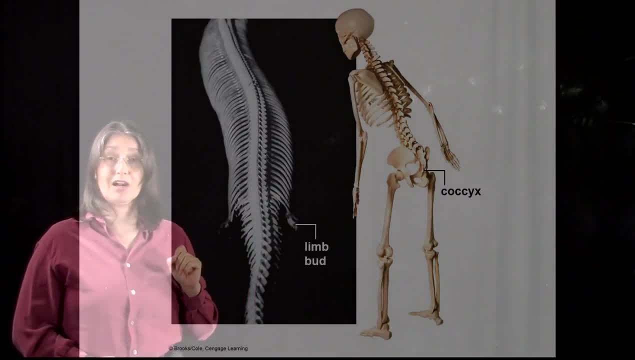 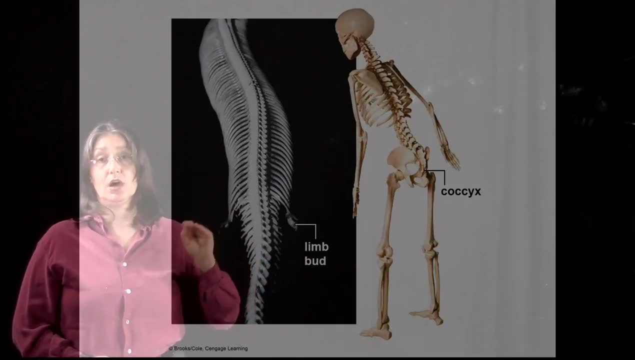 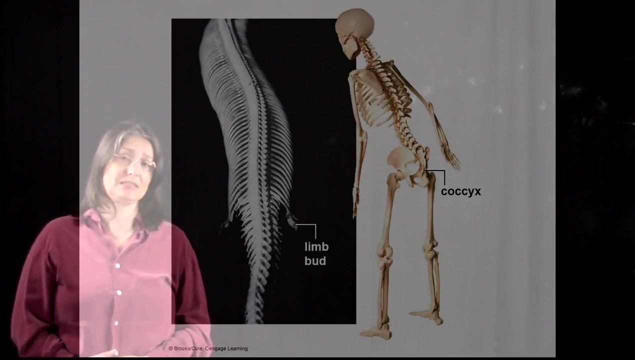 think here you can see the skeleton of a boa constrictor, so a very large snake that even though it doesn't have legs, it does have remnants of legs, at least in its skeleton. So look into this idea of vestigial structures and from the study, 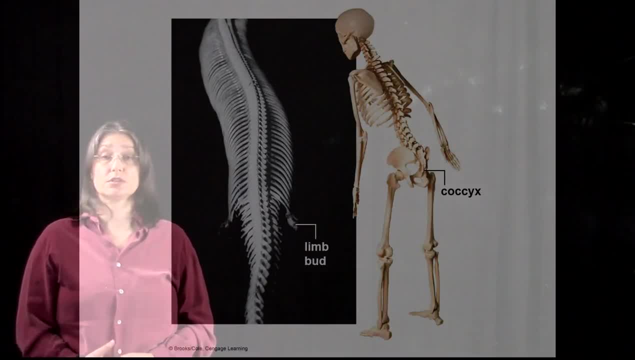 of embryology. you can look into other structures that human embryos have throughout our ontogeny. that it's considered to be a quick summary of phylogeny. So what are these big words mean? What is ontogeny versus what is phylogeny, and what are some examples of vestigial characteristics that we might? 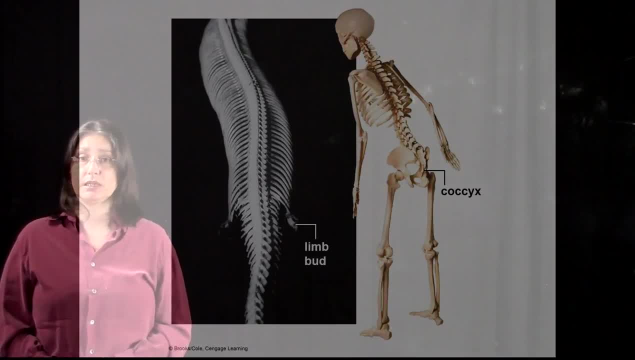 still have And are these vestigial traits or vestigial structures just useless and can only lead to infection, surgery and potential death, such as the appendix, which is considered a vestigial structure, Or some of them. gain new value. they gain new functions. 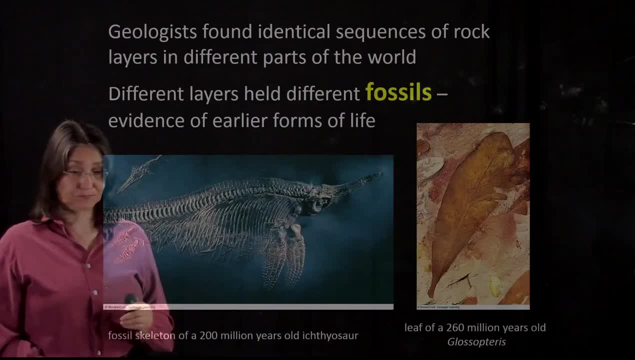 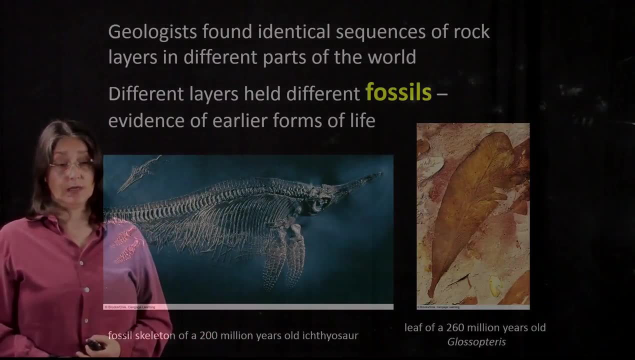 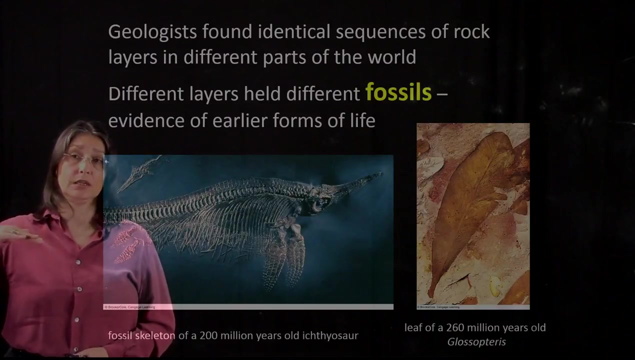 So take a look into this idea of vestigial characteristics. So, moving on to the next area of naturalist explorations, geology was crucial into understanding evolution And, besides, the fact that geologists realized that if you go at relatively same depth in 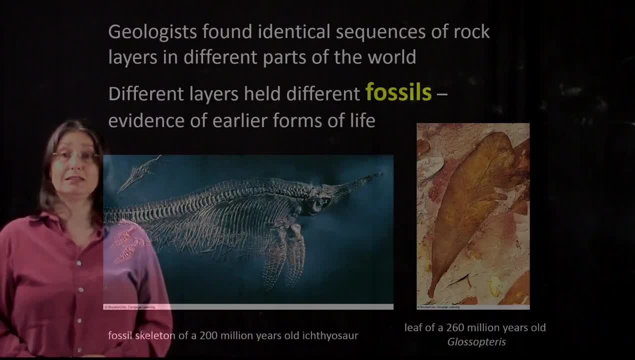 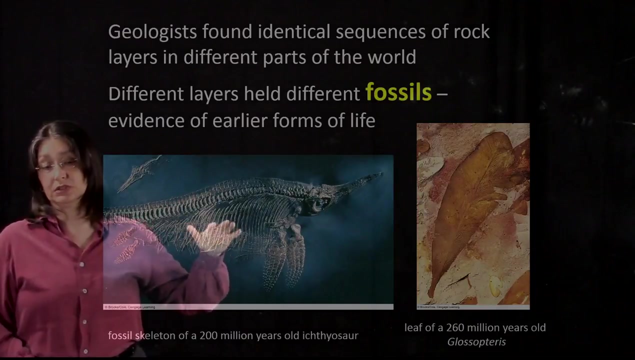 different areas of the earth, you will find similar types of rock And while digging for this similar type of rock, geologists and ecologists and paleontologists have discovered fossils And, as I mentioned before, fossa in Greek means hole. So these are remnants preserved, either a whole skeleton in the case of this, 200 million. 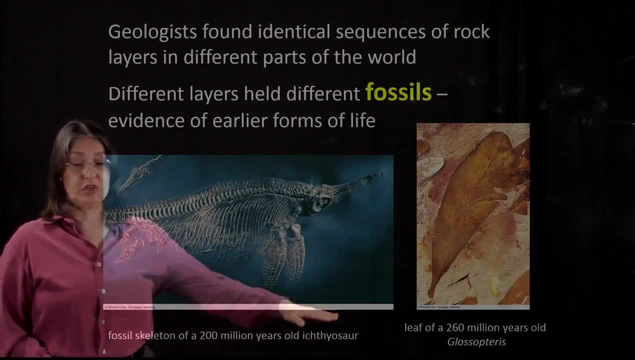 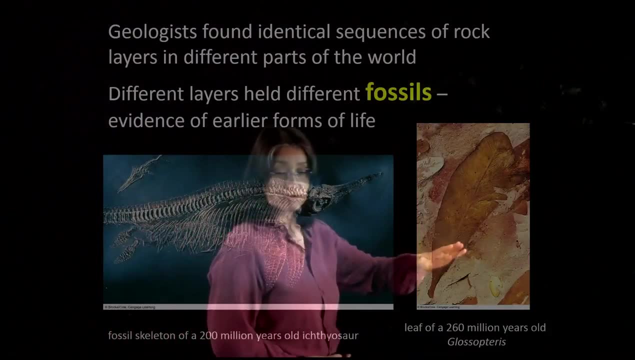 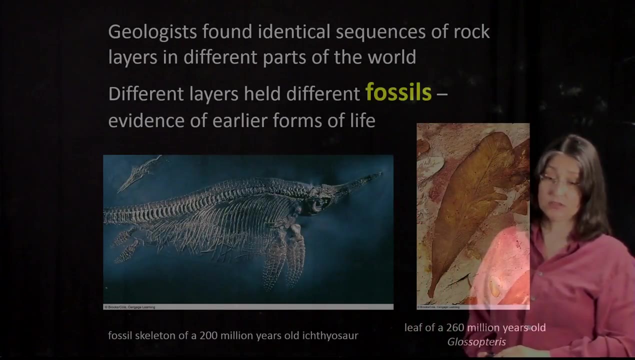 years old Ichthyosaurus, or literally a fish lizard, or just impressions in rocks of organic structures that preceded this impression, this fossil. So this is a fossil of a leaf that was labeled glossopteris, And the name it's relatively simple: glossa means tongue, in Greek. 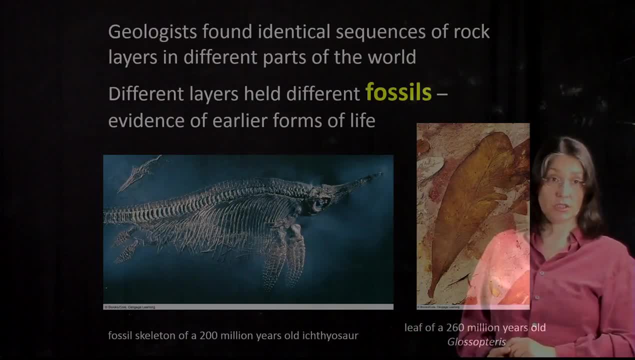 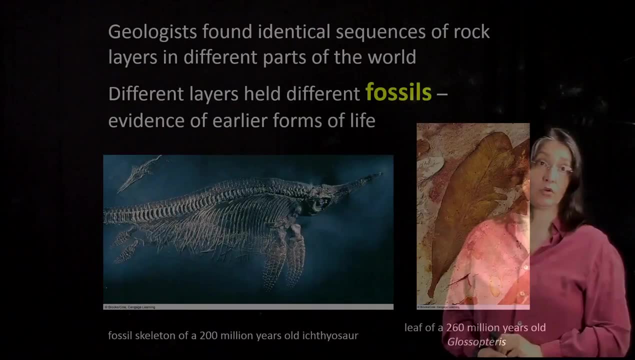 That's why we still have the word glossary, which is a mini dictionary, at the end of most books, including your textbook, So check it out whenever you have a question about the origin of a word or what does that word mean. Pteros means wing. 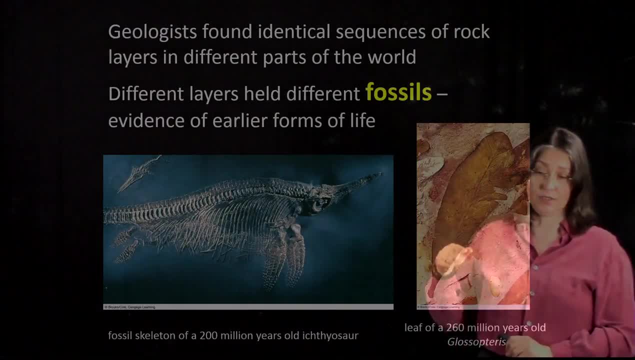 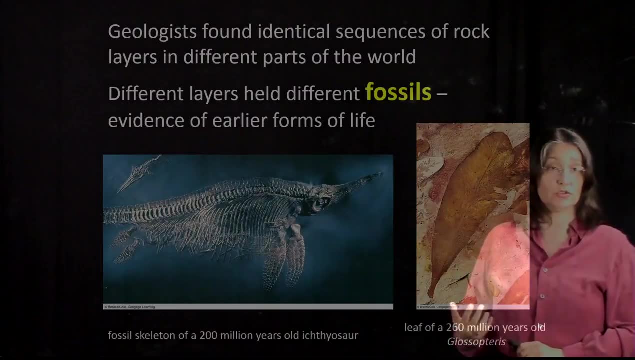 So the shape of this leaf would look like a tongue, but because of the veins, so the midrib and then the lateral veins of this leaf could look like a feather as well. hence the name glossopteris. But speak about fossils. 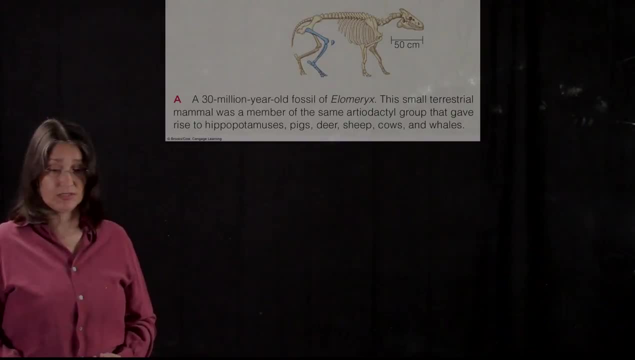 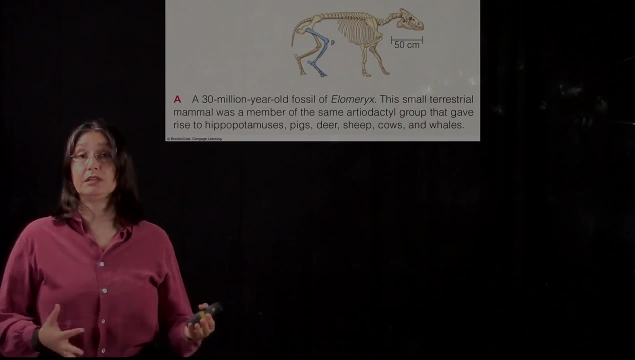 Because of the study of fossils and paleontology. now we know that, believe it or not, whales are, I don't know. They are beautiful, They're very beautiful, And they have their own evolutionary origin and a common ancestor on land. 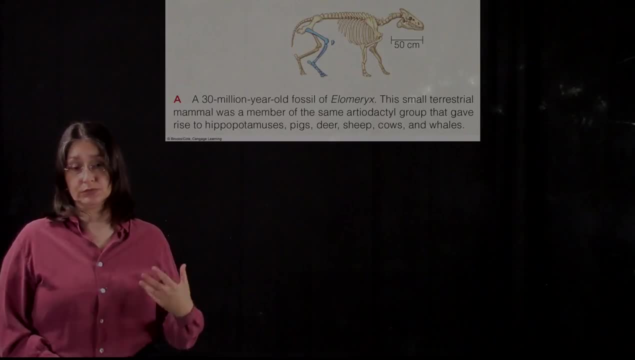 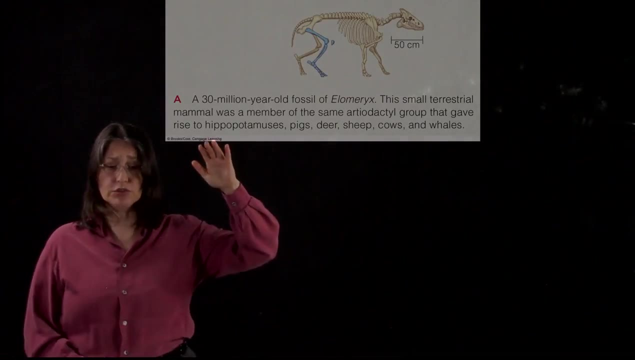 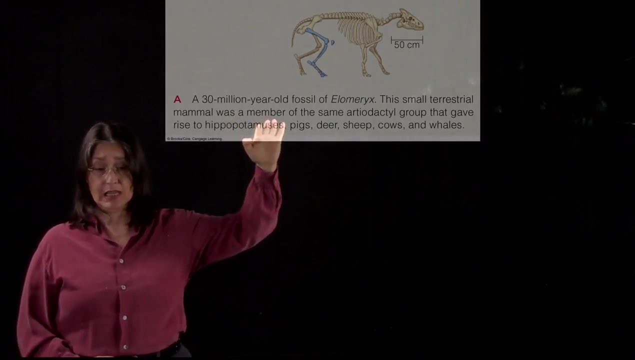 So this is a fossil that's probably related to a group of four-legged or tetrapods that includes hippopotamus, but also pigs, deer sheep, cows and whales. So if you look at the name again, in Greek hippopotamus literally means river horse. 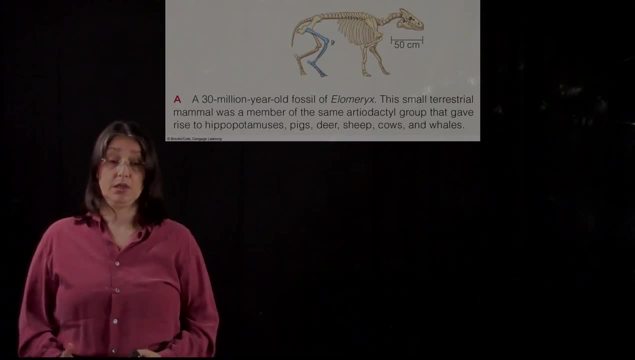 So it's a name that you can use. It's a good name- river horse- because they do so. they are large herbivores that are actually submerged in water for a long period of their time. So that makes the connection in between them.